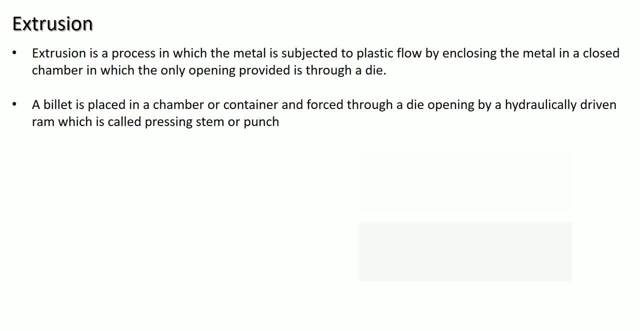 opening provided is through a die. A billet is placed in a chamber or container and forced through a die opening by a hydraulically driven ram which is called pressing stem or a punch. So, friends, extrusion is a process where the billet, billet, it is nothing but the raw material. 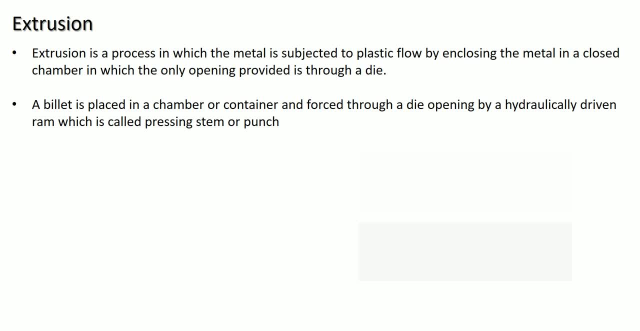 raw metallic material which will be kept in a container, and with help of ram, which is also called pressing stem or punch. with the help of that ram, the pressure is applied on that raw material which is placed in the container. and to that container, one opening will be provided. The shape of, or the cross section of, the opening will be such that 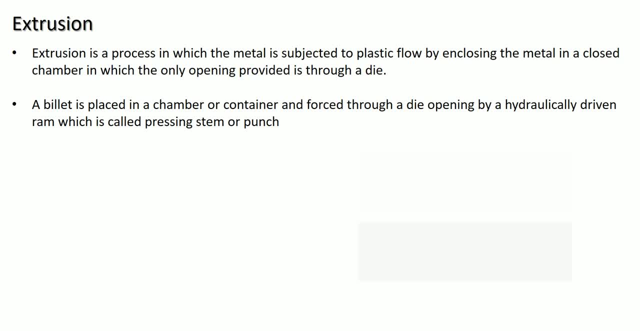 which will be the cross section of the required product. So when the pressure will be applied, the raw material which is kept in the container, the material will come out from that opening which is having desired cross section, That opening, it is nothing but the die, Through that die, the material. 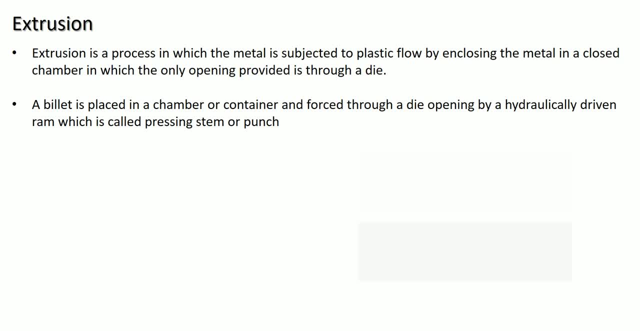 will come and when the material will come through that die, it will acquire the cross section or the shape of that die. and by acquiring the shape or the cross section of that die by the material that will be the that will be nothing but the required product. So in this way, in the extrusion, 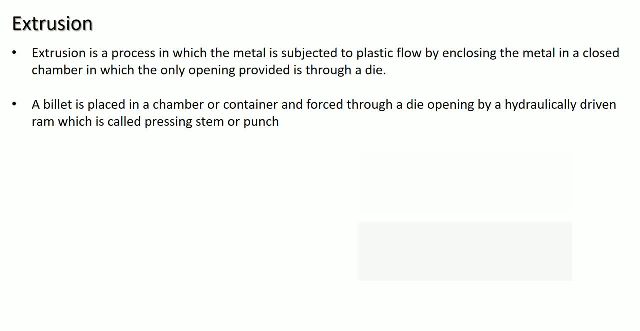 process, by applying force on the billet so that the material will, or the billet will come out from the die and that come out material which will be nothing but the required product. So in this way, with the help of extrusion process, the production or the metal formation process, it is carried out. 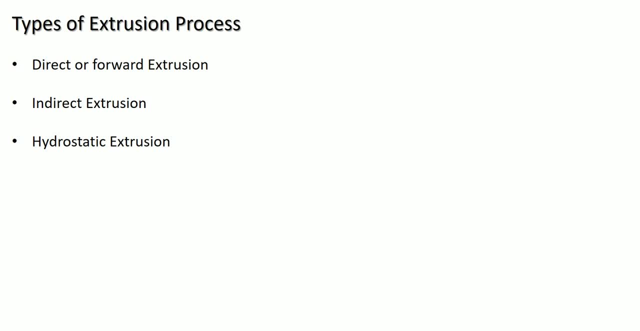 Now let us see the types of extrusion process. Basically, there are three types of extrusion processes. Number one, direct or forward extrusion. number two, indirect extrusion. and number three, hydrostatic extrusion. Now let us see all these three types one by one in detail. First one: 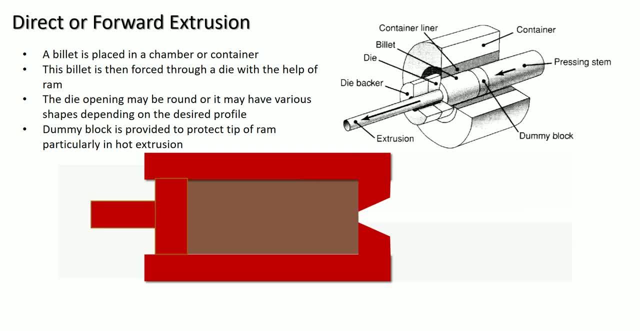 direct or forward extrusion. In the direct or forward extrusion, a billet is placed in a chamber or container. The billet is then forced through a die with the help of ram. The die opening may be round or it may have the various shapes depending on the desired profile. Dummy block is provided. 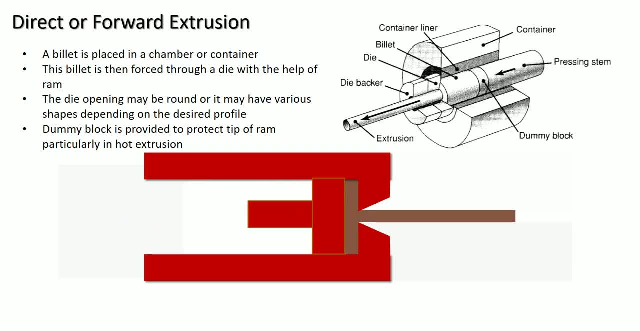 to protect the tip of ram, particularly in hot extrusion. So here we can see the diagram of direct or forward extrusion. Here we can see that this one is the billet which is kept in the container and this one is the pressing stem or 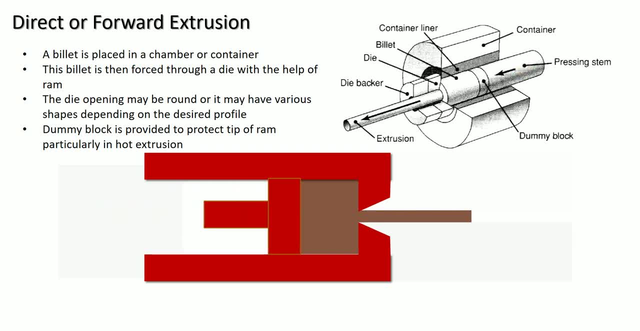 it is also called ram. So with the help of this ram, the pressure will be applied on this billet, and this one is the opening which is called the die of this container. So when the pressure is applied on on this billet with the help of this pressing stem, whatever the billet is inside there, 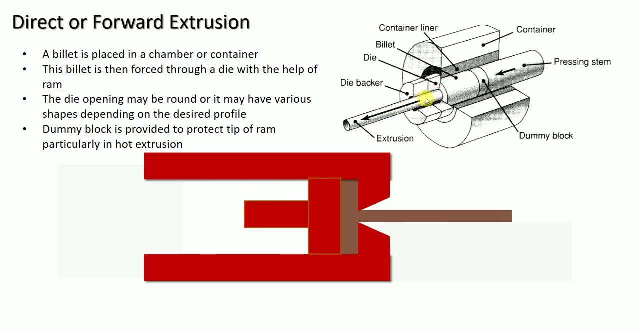 that billet will come out through the opening which is kept in the container. Now let us see what is called the die and at the time of coming out this material, it will acquire the shape of this die. So that means whatever the desired shape we want, that will be acquired when the material. 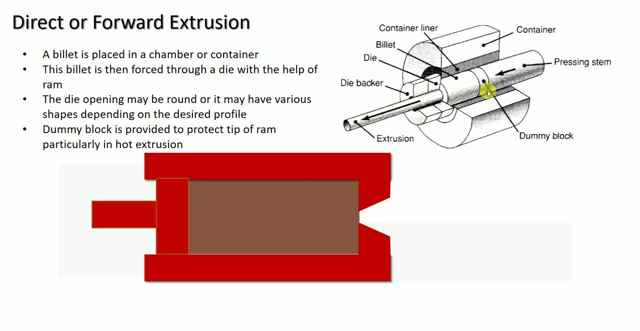 will come out through this die. Now, here, in between this billet and pressing stem, one object is there which is called dummy block. So the function of this dummy block is it protects the pressing stem from, we can say, erosion. So basically it is used in the hot extrusion process. 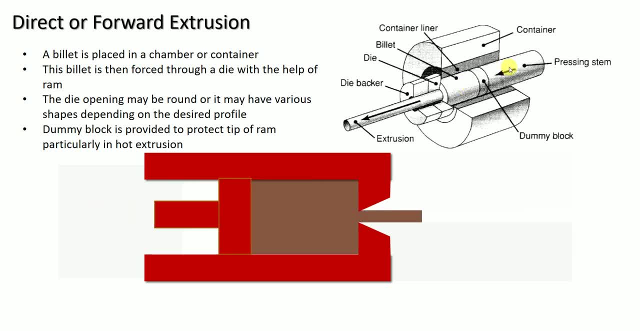 as the temperature of this billet. it is very much high as compared to temperature of this pressing stem. In order to protect this pressing stem from this high temperature, it is used Now. here we can see the animation of this direct or forward extrusion process. We can see that this one is the 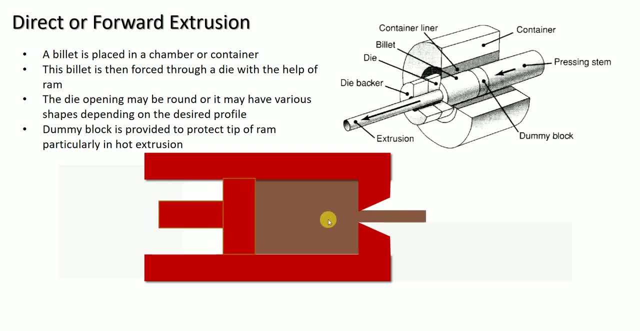 pressing stem and this one is the billet when the pressing stem, when that ram will apply the pressure on that billet, at the same time that billet will come out through this opening which is nothing but the die. and at the time of coming out from this die, by this billet, it will acquire. 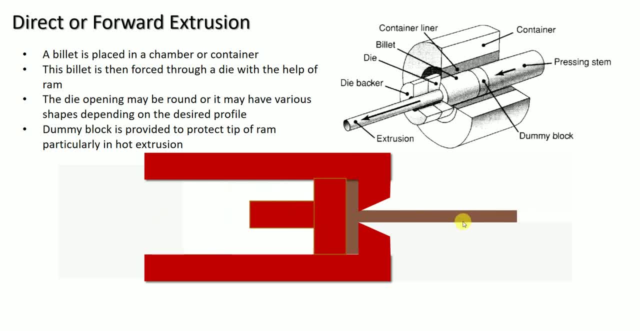 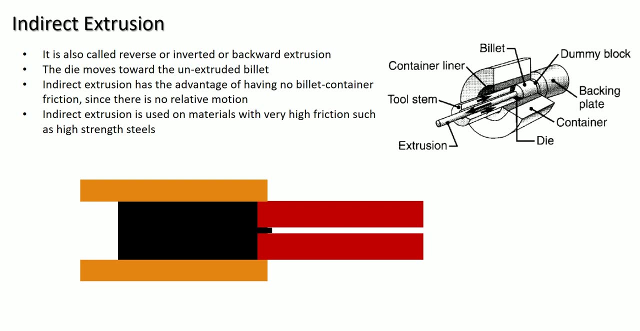 the shape. So here we can see that this one is the extrusion obtained here. Now let us see the second type of extrusion process, indirect extrusion. So in the indirect extrusion process it is also called reverse or inverted or backward extrusion. Here the die moves. 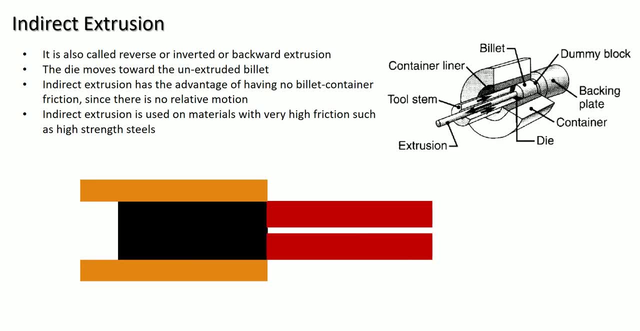 towards the unextruded billet. Indirect extrusion has the advantage of having no billet container, since there is no relative motion. Indirect extrusion is used on the material with very high friction, such as high strength steel. Here we can see that the diagram of this indirect extrusion 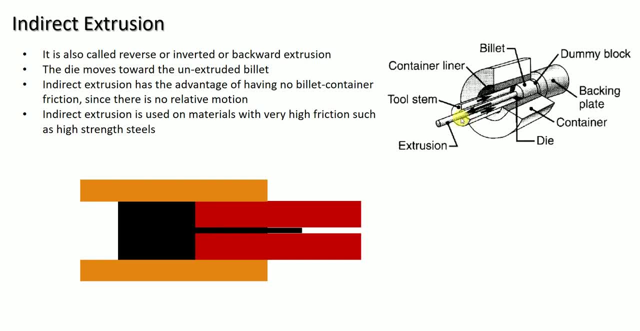 process. Now here the movement of this pressing stem or ram. it is towards the unextruded billet. So here we can see that this one is the pressing stem and it is moving in this direction. and when this pressing stem is moving in this direction, 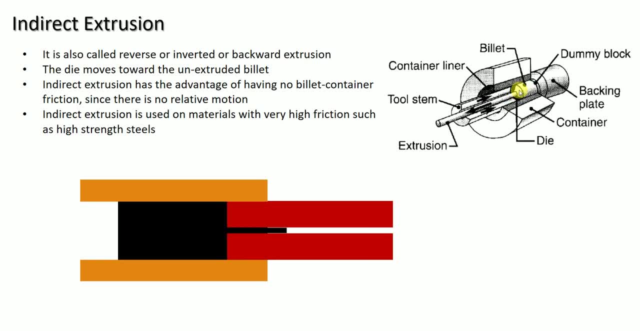 at the same time, this billet extruded billet. it is coming out in the direction which is exactly opposite that of the pressing stem. So pressing stem is moving in this direction and billet is coming out through the die in the reverse direction. So when the pressing stem will apply. 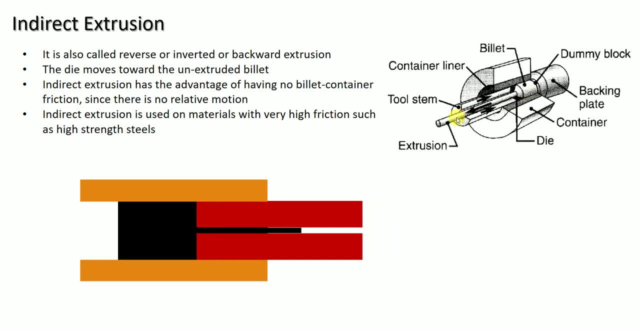 the pressure. This means that the die is on this billet and at the pressing stem itself it is. it has given the opening. So that means the die is provided on the pressing stem because of the application of this pressure by the ram. the extrusion will be carried out there and this billet will be coming out. 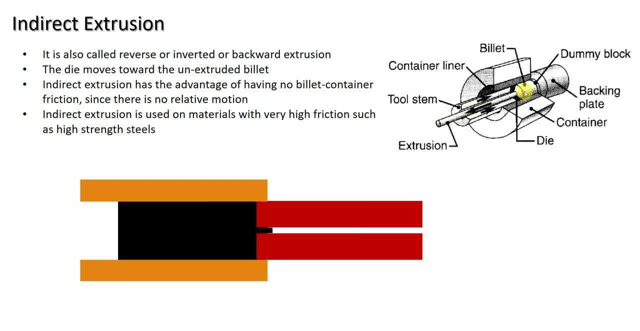 through this die. Here there is no movement of the billet like in the direct extrusion process. We have seen that when the pressure will be applied on this billet by the ram, the movement of that billet it is taken place. So such movement it is not here in case of. 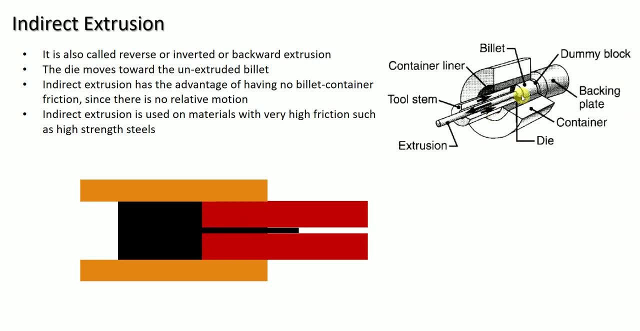 indirect extrusion. So, because of not having the movement of the billet, there is no friction in between the container and the work piece. So because of which, the container, it is protected, because of no friction. Now, this, this process, or the indirect extrusion process, because of no friction, it is generally. 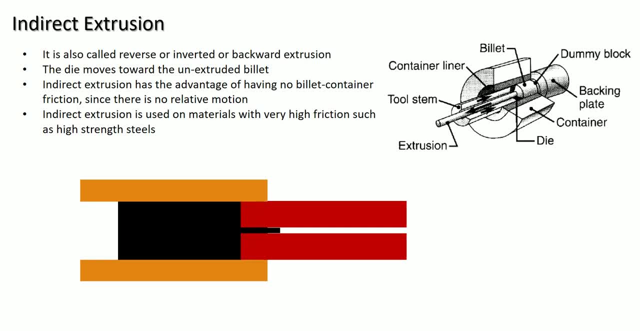 used in the material which which is having very high coefficient of friction, such as high strength steel. Here we can see see that the animation of indirect extrusion process. So here we can see that this one is the ram and this ram it is applying pressure towards the billet side. 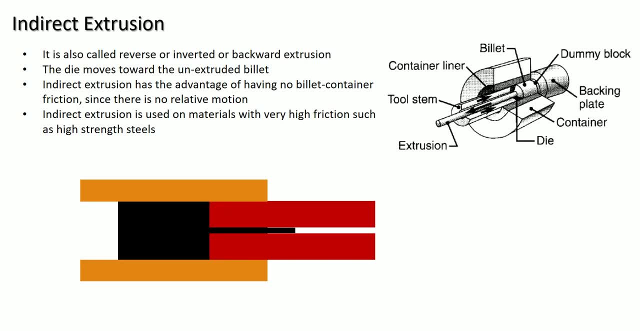 unextruded billet side And because of the application of the process, the extrusion process, it is carrying out in the reverse direction. That means here we can see that the extrusion is carrying out in this direction and billet is moving in this direction. So in this way the indirect extrusion process is carried out. 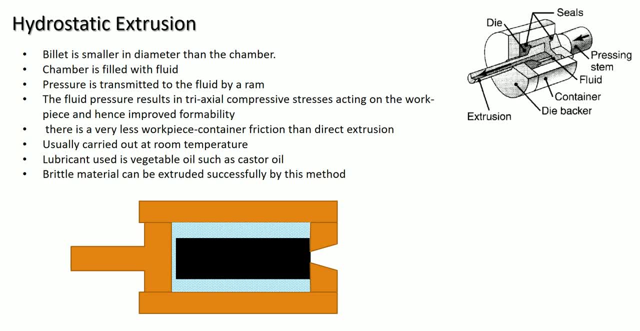 Now let us see the third type of extrusion process, which is hydrostatic extrusion. In the hydrostatic extrusion process, billet is smaller in diameter than the chamber. Chamber is filled with the fluid. Pressure is transmitted to the fluid by a ram. 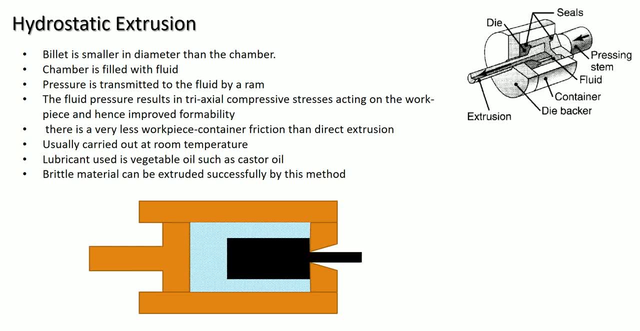 The fluid pressure results in triaxial compressive stresses acting on the work piece and hence improved formability. There is a very less work piece container friction than the direct extrusion. Usually it is carried out at the room temperature. Lubricant used is vegetable oil such as castor oil. 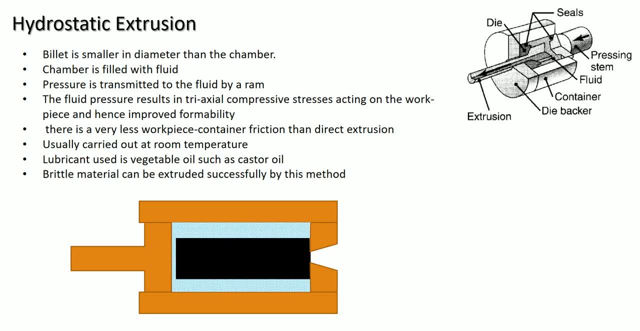 Brittle material can also be extruded successfully by this method. So here we can see the hydrostatic extrusion process. in the hydrostatic extrusion process, As the word hydro is there, that means the fluid will be used here to apply the pressure on the billet so that it will come out through the die as a extrusion. So here we can see that. 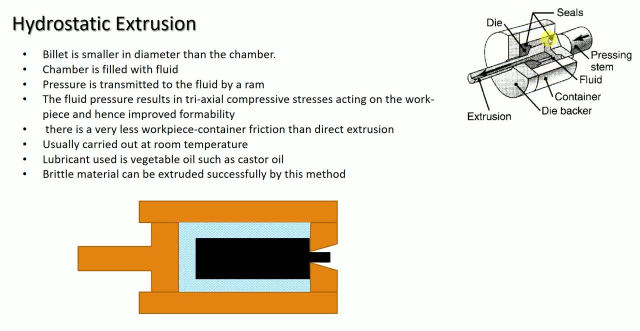 this one is the container and inside the container fluid it is filled. This one is the billet and this one is the pressing stem. When the pressure will be applied by this pressing stem, that pressure it will not be directly applied on this billet. 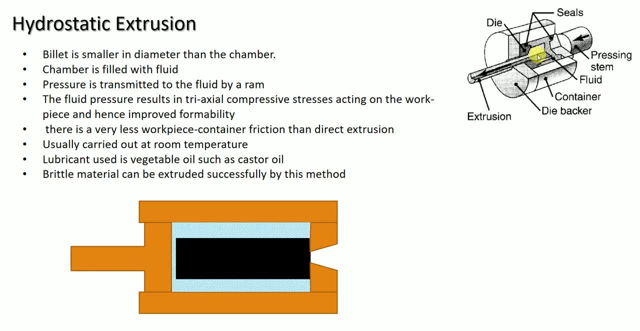 Here we can see that. one thing is there: the size of this billet. it is very much smaller than the size of container. So that means there is this very wide clearance between the billet and this container. Now this one is filled by the fluid When the pressing stem will apply the pressure. 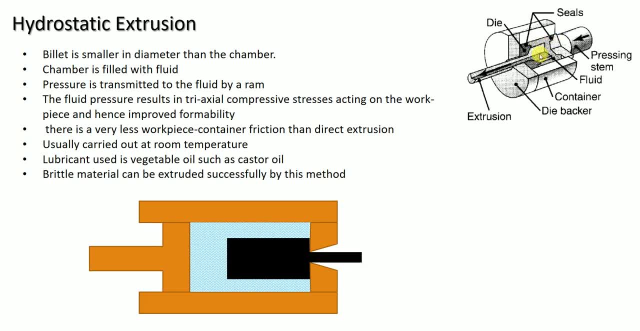 that pressure will be not directly applied on this billet. it will be applied on the fluid which is inside the container and as the pressure will be applied on the fluid that pressurize the fluid, it will apply pressure on this billet in all the three directions, So that means triaxially this. 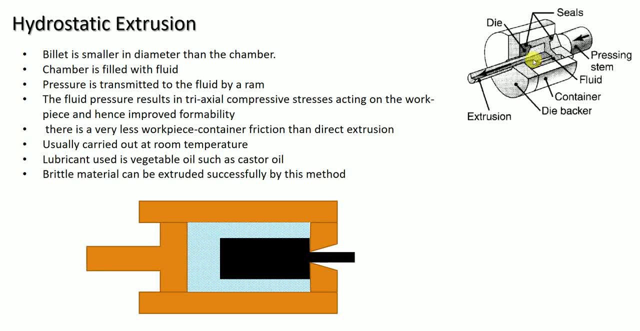 fluid will apply pressure on this billet and because of the application of this pressure by the fluid on this billet, the extrusion process it is carried out Now here, as the fluid we are using to pressurize the fluid, there will be no friction like in the 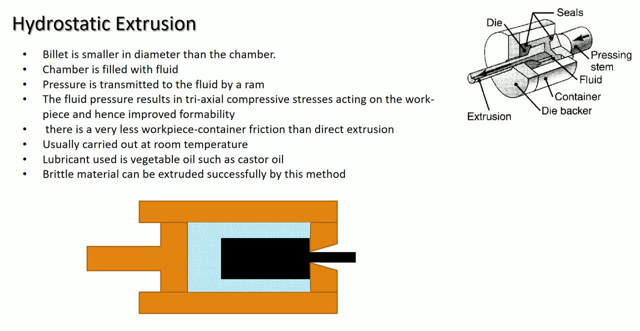 direct extrusion process. Here we can see the animation of this hydrostatic extrusion process. Here we can see that this one is the fluid contained in the chamber, or the container. This one is the ram. Now, this ram, it is applying pressure directly on the fluid, not on the billet Because of the 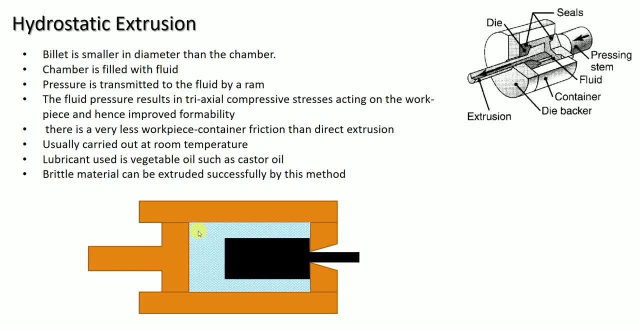 application of pressure on this fluid. fluid is pressurized and it is applying pressure on this billet And because of application of pressure on this billet, the extrusion process it is carried out. Now here we can see that there is a very large gap in the 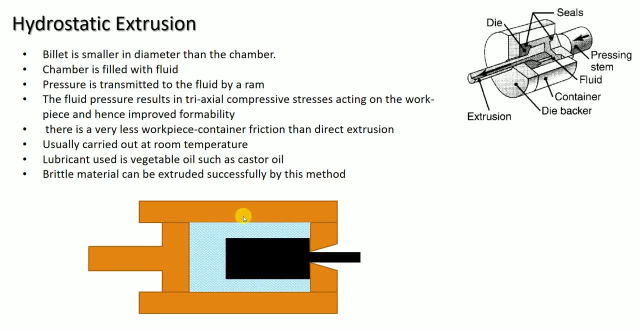 between the billet and this container. so that means there is no direct contact between this billet and container. there will be no friction like direct extrusion process. so this is one of the major advantage of this hydrostatic extrusion process. so, friends, in this way, in this video, we